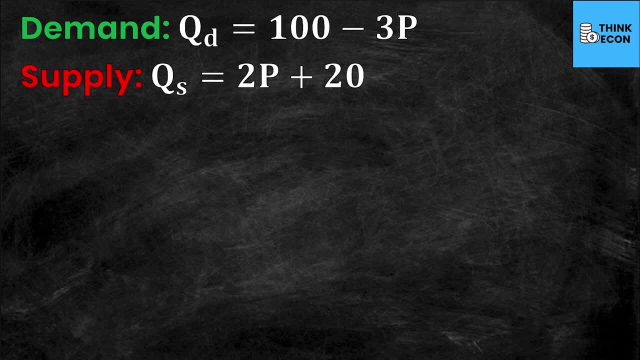 demand curve and the supply curve intersect. However, for some reason, you don't want to actually draw out the two curves. Well, you can do all of this algebraically and it's quite simple. Now remember: in equilibrium, quantity demanded is equal to quantity supplied, So the two lines. 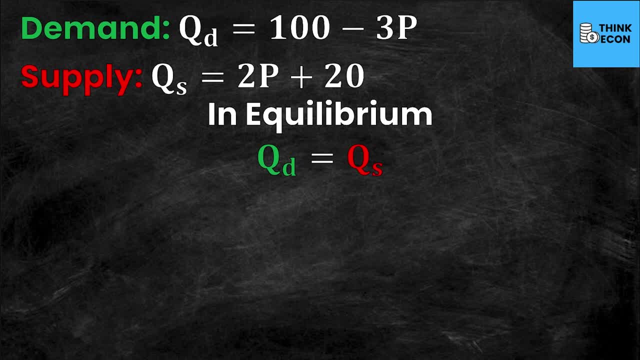 are intersecting and their q value and their p value is the same, So we can take this bit of knowledge and use it to solve this equation. Now let's say that we have a supply and demand curve, So we have: qd is equal to qs. Now I have quantity demanded in green and quantity supplied. 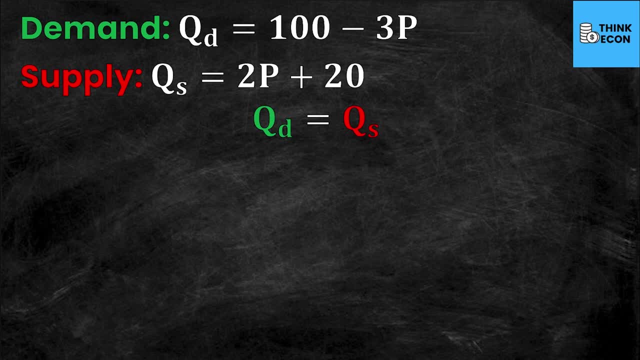 in red, just so you can tell them apart. However, I will lose the colors in a bit, so bear with me. here I have: 100 minus 3p is equal to 2p plus 20.. And, as you can see, based on my colors, those are. 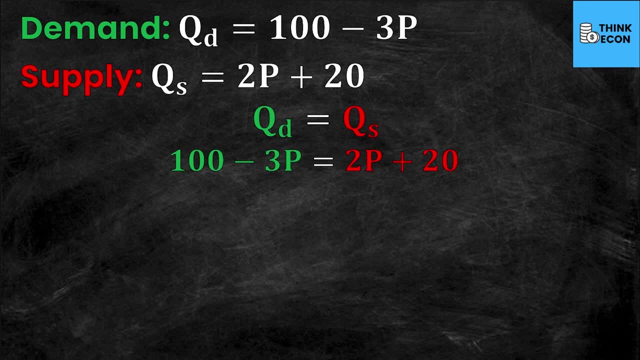 just the quantity demanded and quantity supplied, equations subbed in on either side of the equal sign, since we know, at equilibrium the two qs are actually the same. So I went from having two equations and then I went from having two equations, and then I went from having two. 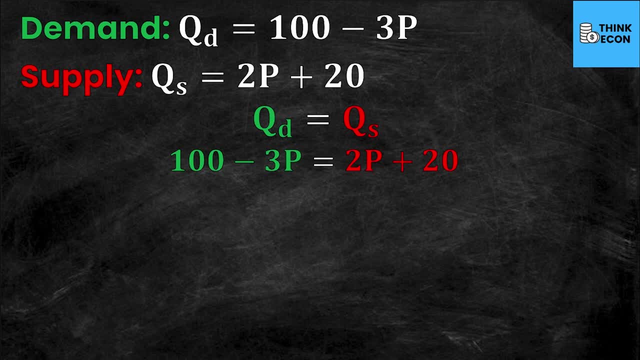 equations with two unknowns to having one equation with one unknown, And the unknown in this case is p. So now I'm going to solve for p, which is the equilibrium price. Now I'm going to collect my like terms on their respective signs of the equal sign. So I'm going to put all of the p's. 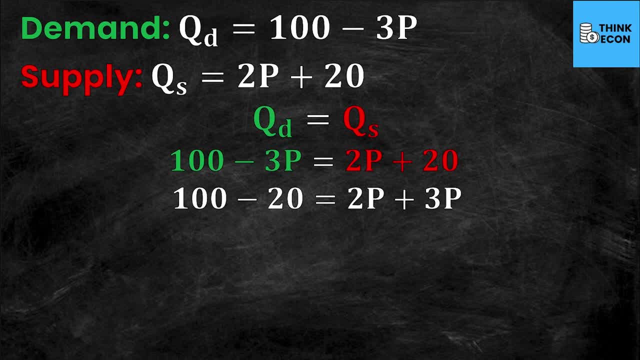 on the right and all of the constants on the left. So I move that positive 20 over to the left side, which is now a negative 20.. And I move that negative 3p to the right side- Now it's a positive. 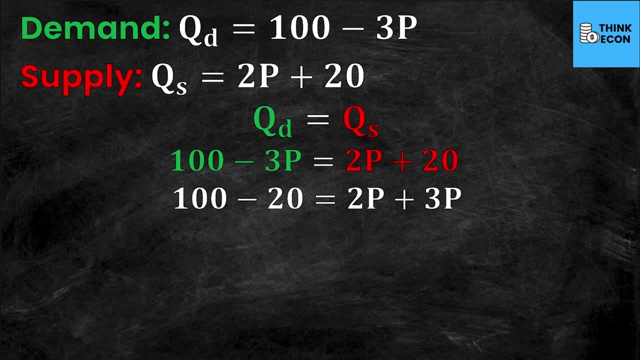 3p. This results with 100 minus 20 is equal to 2p. So I'm going to put all of the p's on the right. this equal to 2p plus 3p. With more simple algebra, I'm just going to solve those two lines. 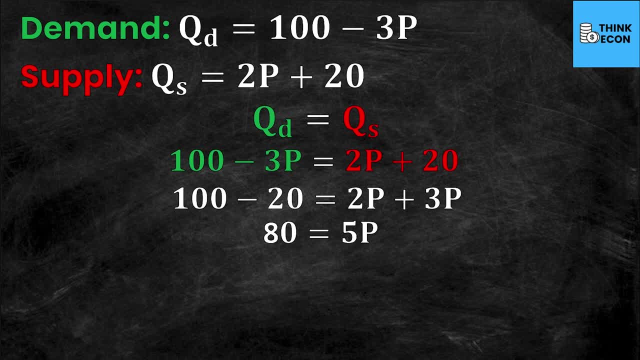 100 minus 20 is 80. And 2p plus 3p is simply 5p. Now I want to isolate p, So I'm going to divide both sides by five. 80 divided by five is 16.. And 5p divided by five is just p. So now I have. 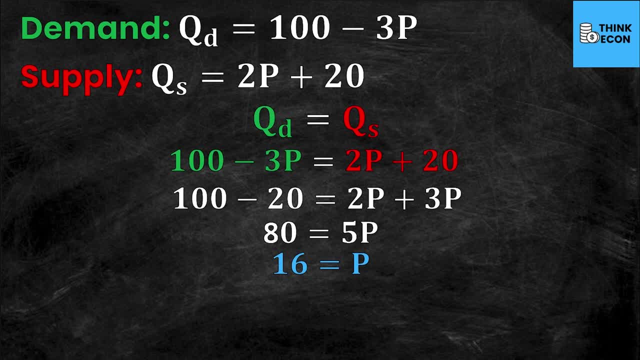 16 equals p, And if you're like me, I like to have the letters on the left side. that's more of a mental thing than anything. So I've also written: p is equal to 16.. That is my equilibrium price. Cool, But how do I use the equilibrium price to solve for the equilibrium? 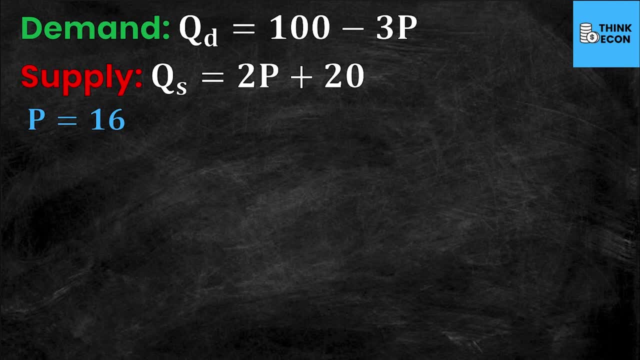 quantity. Well, we did say at the very beginning that qd is equal to qs, which means technically I can take that p equals 16 and sub it into either equation. And to show you that's going to work, I'm going to sub it into both equations in this video And you'll see that it yields the exact 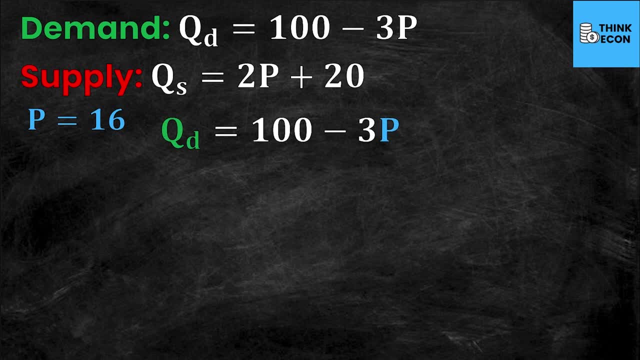 same equilibrium quantity. So first we're going to sub it in to quantity demanded. So quantity demanded minus 3p- But we know what p is, So we're going to sub it in- Quantity demanded is equal to 100 minus 3 times 16.. 16 is just my equilibrium price which I calculated earlier. Now I have 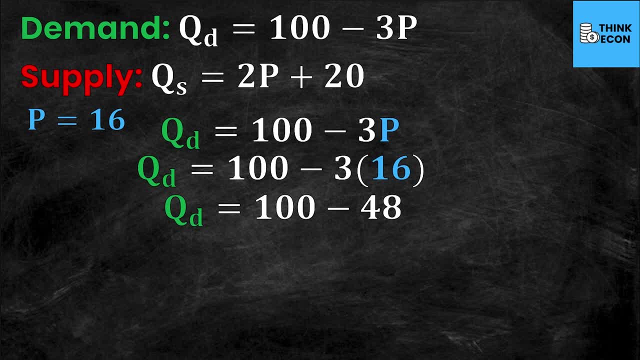 that quantity demanded is equal to 100 minus 48.. 48 is simply 3 times 16. And then, with some simple subtraction I'm going to have: quantity demanded is equal to 52.. Now, that was me subbing in 16 for. 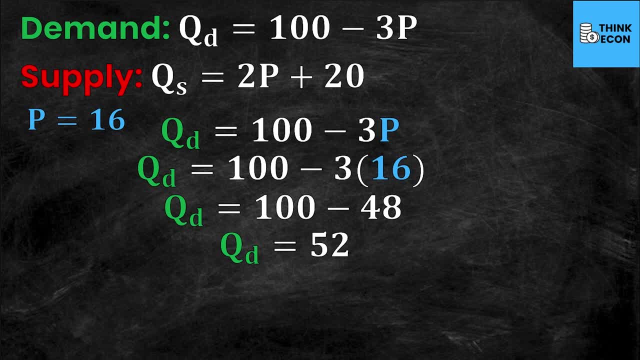 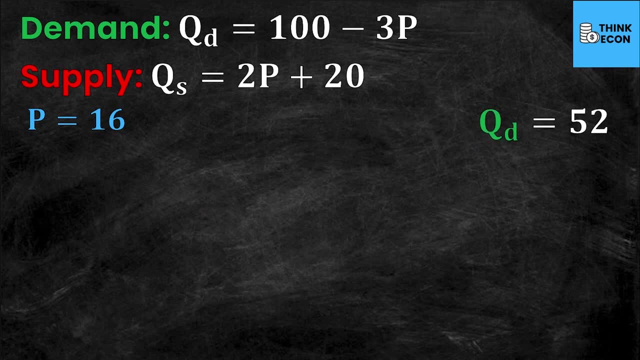 p in the demand equation, But I was telling you- I'm going to sub it in to quantity demanded- that you would get the exact same result if you subbed it into the supply equation. So let's do that now, just to make sure that we have our algebra correct. So let's pull up our quantity. 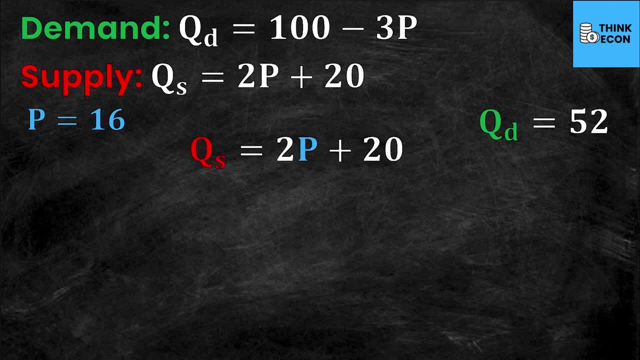 supplied equation: qs is equal to 2p plus 20.. Now again we know what p is: It's 16,, just like it was before. So now we have: qs is equal to 2 times 16 plus 20.. Well, 2 times 16 is simply 32.. And 32? 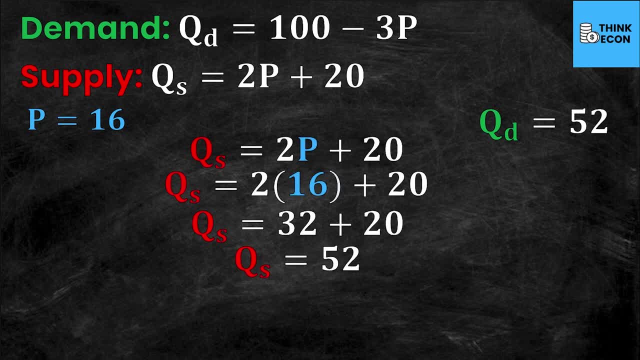 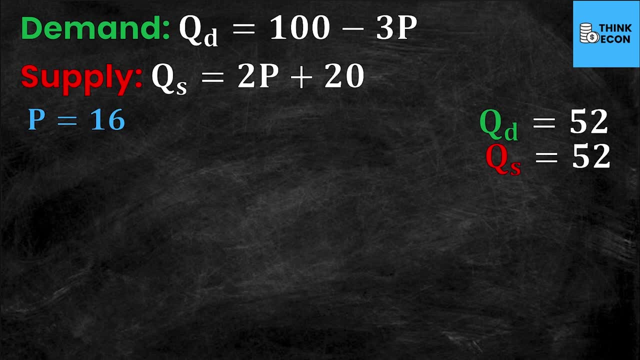 plus 20 is equal to 52. So now we've derived that quantity supplied is also equal to 52. And that's exactly what we expected, since at equilibrium the two quantities, quantity demanded and quantity supplied, should be the same. So now we have: qs is equal to qd. 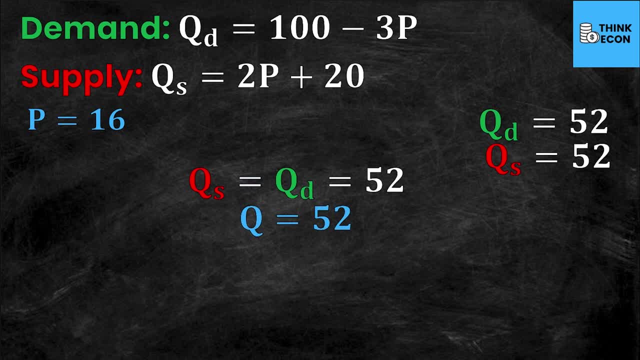 which is equal to 52.. And this means that q at equilibrium must be equal to 52.. And you can see my two equilibrium values on the slides in blue. So now I have my equilibrium p, my equilibrium q, And if I wanted to, I could write them out as a point. 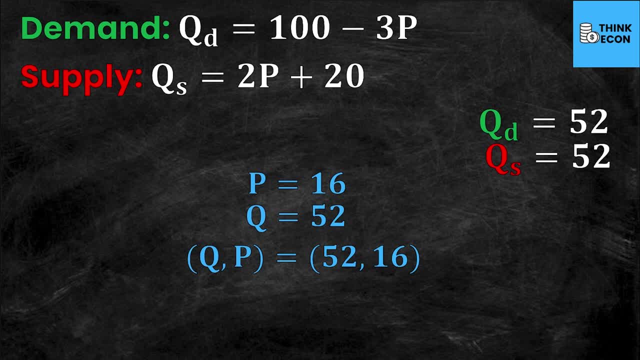 That is my point on a graph. that is my equilibrium quantity and price. However, you might have learned- and this is something that I teach my students- that you want your p and your q to be. you want to denote them as equilibrium points, Because right now I just have, p is equal to 16,. 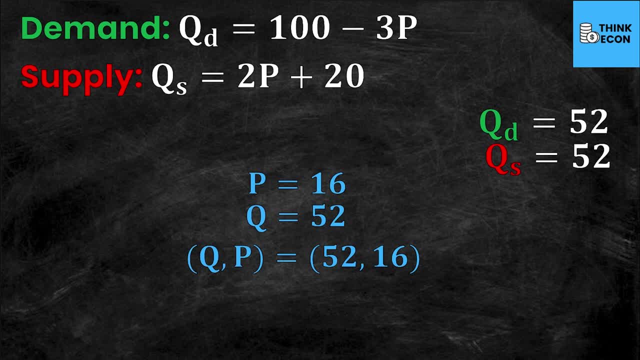 but that doesn't tell me it's equilibrium price, It doesn't tell me that it's equilibrium quantity. So what I like to do, and I teach my students to do, to add a star or an asterisk, which will give me a point that is equal to 16, q star is equal to 52.. And that just means p star and q star are 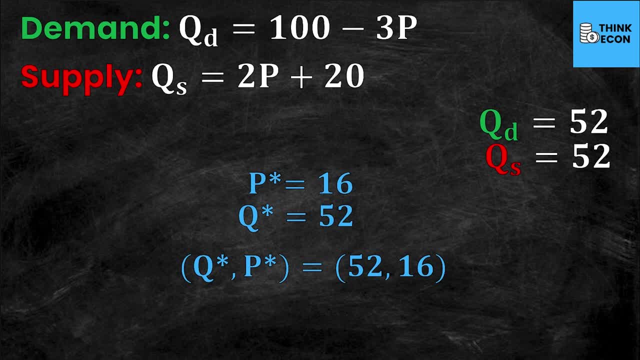 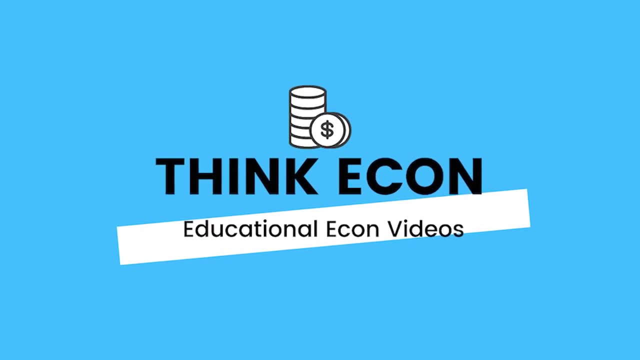 your equilibrium values. That way you don't confuse them. for a different point that is a different p and a different q. So there you have it. Now you know how to use simple algebra to solve for equilibrium price and quantity without actually having to graph the supply and demand curves. 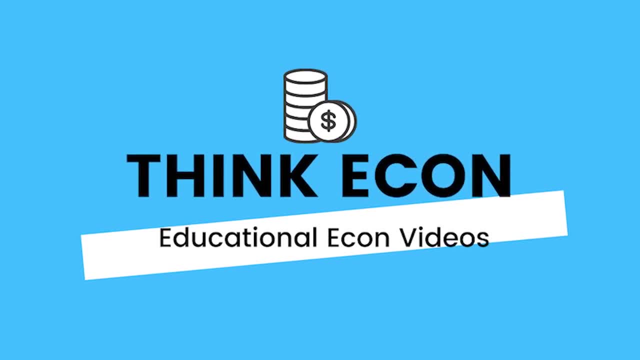 yourself. If you found this video helpful, let us know by liking the video, subscribing to the channel and, of course, leave us a comment in the comment section below. Thanks for watching this video and we'll catch you in the next. Thanks for watching. 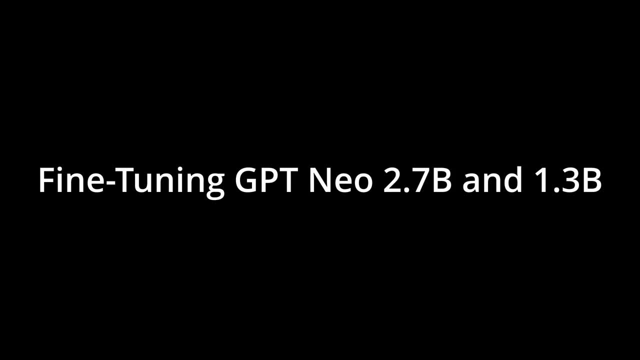 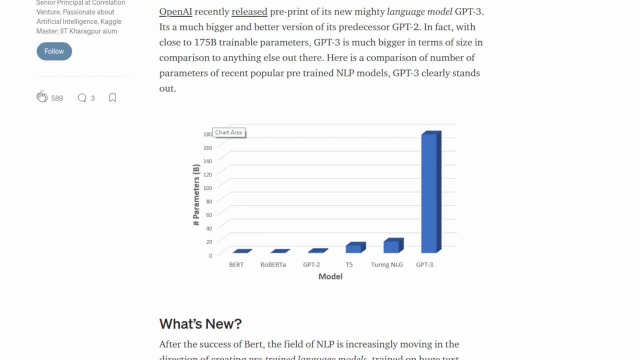 What's up guys? Today we're going to be going over GPT-NEO, the open source implementation of GPT-3. If you recall from my previous videos, what makes GPT-3, and to a lesser extent, GPT-NEO so special, is the vastly increased size. Here's GPT-3, here's GPT-2. At this time, the largest GPT-NEO model is 2.7 billion parameters. 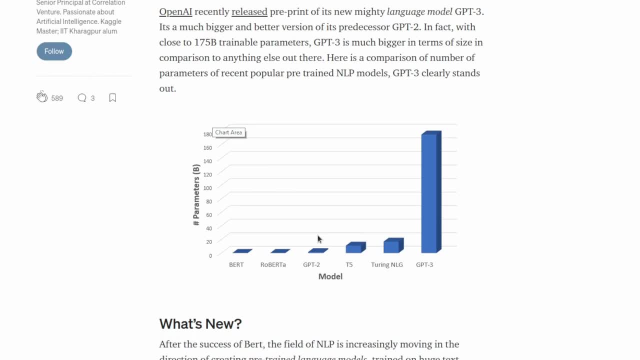 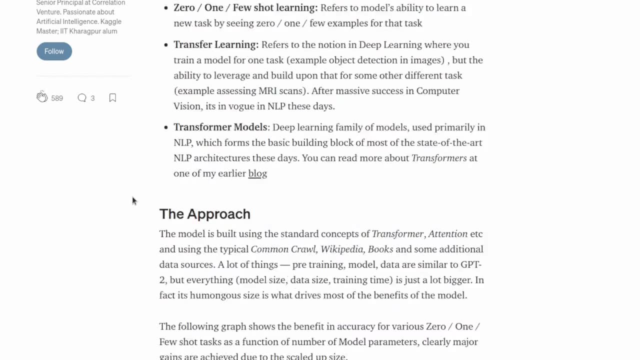 While this is still much smaller than 175 billion parameters, having a larger model has its benefits. Specifically in the area of fine-tuning and few-shot learning. 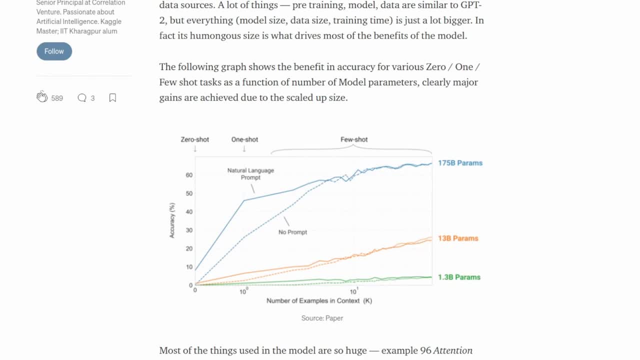 What we see in this diagram here is the ability of different size models on their impact of learning from one-shot, zero-shot, and few-shot. What this means is how many examples is a model being given to complete a specific task. 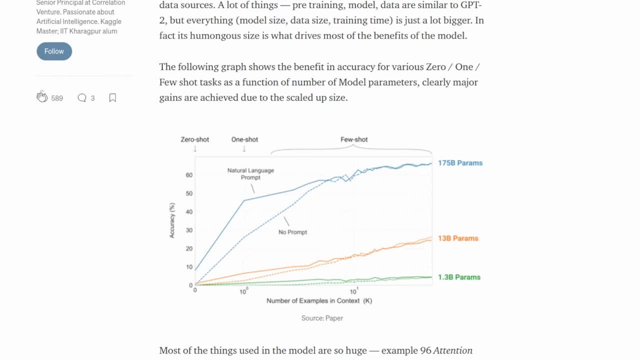 Sentiment analysis of text, and text generation in a certain style, such as generating text in the proper format of a programming language. What we see in this diagram here are three models, 175 billion parameters, 13 billion parameters, and 1.3 billion parameters. 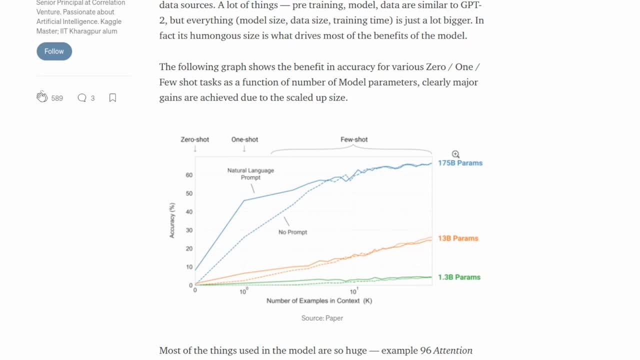